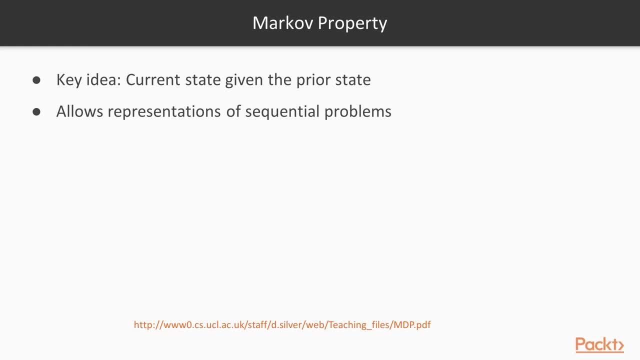 This is useful for RL because RL often deals with sequential problems. More formally, the probability of state S at time t plus 1 given state S sub t is equal to the probability of S t plus 1 given all prior state history. Next we'll go over key MDP terminology. 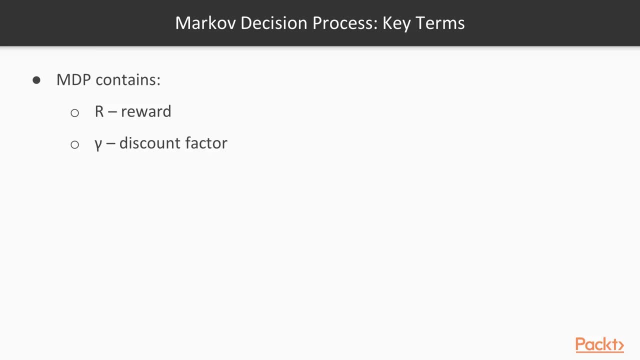 MDPs contain reward R, discount factor, gamma actions, A, state transition probabilities, P, R and state S. In the context of MDPs, the reward R is a scale where it receives by transitioning to a state. The return g is the sum of rewards discounted from the current time, step t. 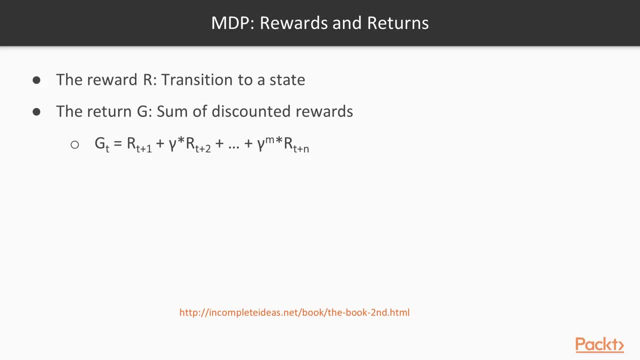 The formula for G sub t is R T plus 1, plus gamma times R T plus 2, until the end of the return μαι. Gamma also makes the math more convenient. Gamma is in the 0 to 1 range, with 0 meaning. 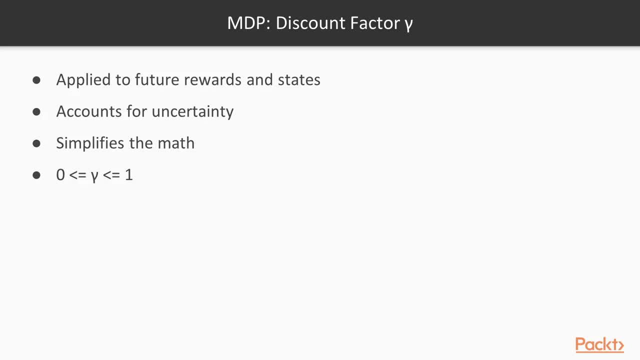 that future states slash rewards are not accounted for, and 1 meaning that future states slash rewards are weighted highly. Gamma less than 1 can be seen as a cutoff For returns far enough into the future. Gamma will effectively be 0, and no returns past. 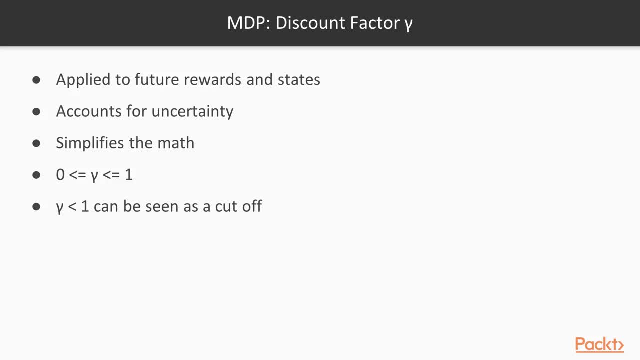 that point will matter. This can help you when choosing what value of Gamma to use for your problem. Consider: how much of the future do you want your agent to account for? The agent can select an action which may result in remaining in the same state or transitioning. 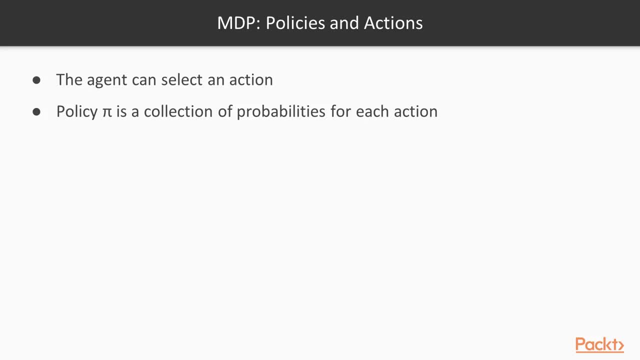 to a new state. A policy pie is a collection of probabilities for each possible action. A state action value can be used to evaluate the goodness of an action given a state. MDPs define that transition probability PR of going to the next state given the preceding. 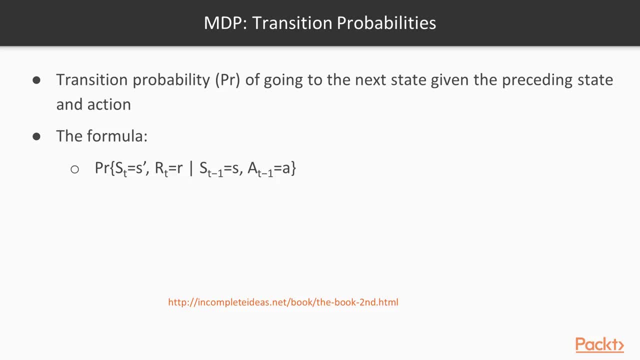 state and action. The formula is read as: the probability of ending up in state S' and receiving reward R, given that the agent took action A in state S. Here is a simple example of the transition probabilities in a Markov process. There are: 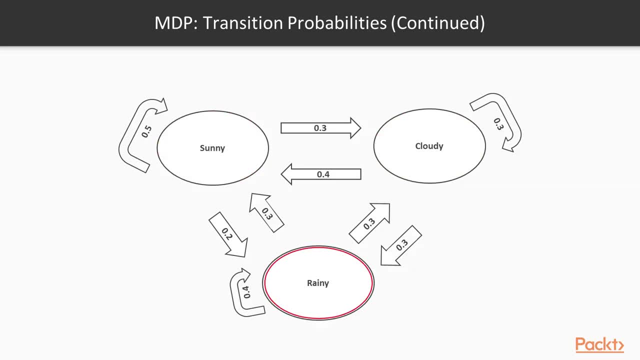 three states: sunny, cloudy and rainy. The arrows represent the allowed transitions and the numbers of transition probabilities. For example, there is a 0.5 chance for a sunny day to remain a sunny day. A 0.3 chance for a cloudy day. 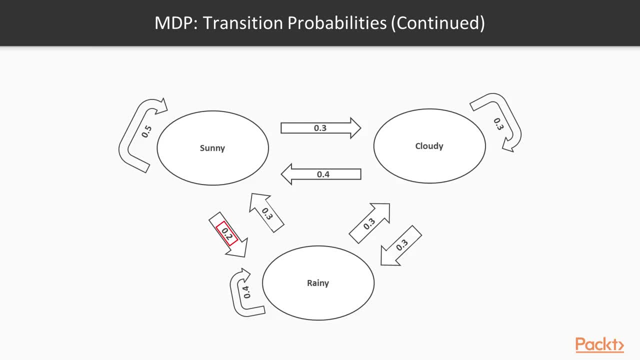 And a 0.2 chance for a sunny day to become a rainy day. Next, we'll add the rewards to the MDP. This is the same example, except rewards are included in the parentheses. For example, if you go from cloudy to rainy, the reward is 0.. If 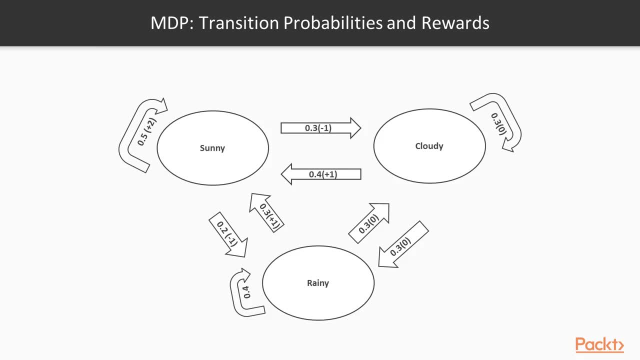 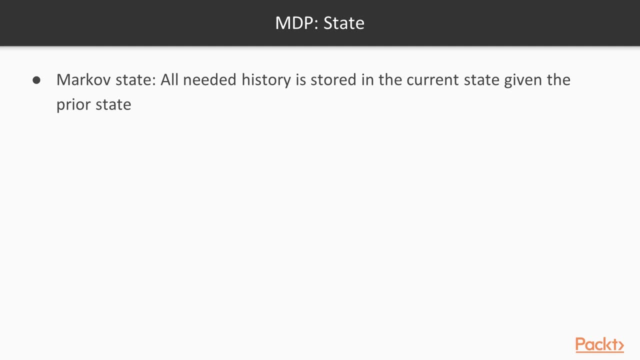 you go from sunny to cloudy, the reward is negative 1. The final term we'll introduce in this video is the Markov state. In a Markov state, all needed history is stored in the current state. given the prior state, Based on the rewards, actions and transition probabilities of the states we can assign, 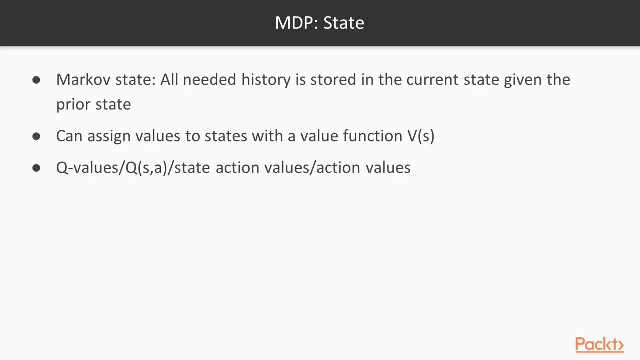 values to the states with the value function Vs. Q values written as Qsa are the state action values, aka action values, Vs values. the state Qsa values the action A taken in state S. Vs and Qsa define the expected value of the state and state-action combination. Vs and Qsa are examples of values that can be used to get a new value. 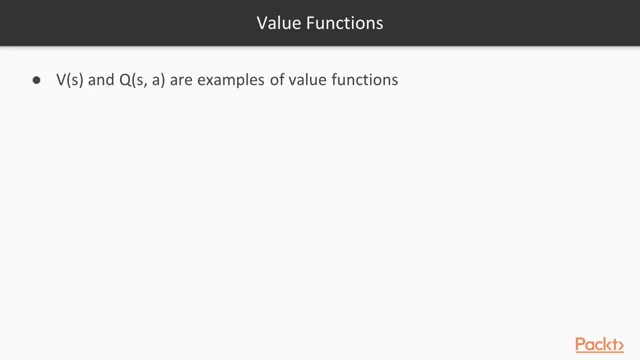 Vs and Qsa define the expected value of the state and state-action combination functions. Value functions are an important concept in RL. Value functions let agents assign a goodness value to states and state-action combinations which help agents determine which states to visit and actions to take. Value functions are based on the expected value. 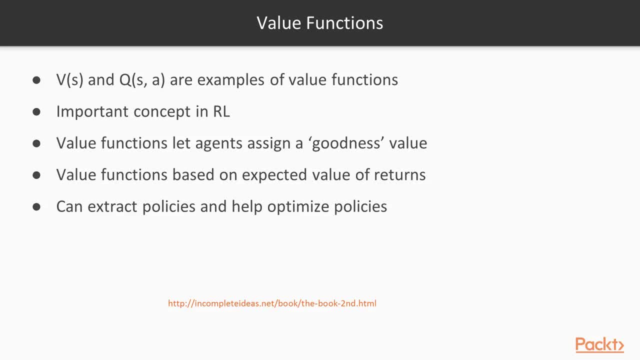 of returns. We can extract policies from value functions, as we'll see in this section, in Section 3's DeepQ Network videos, or use value functions to help optimize policies, like we'll do in Section 4.. Here's an example of the MDP framework with state values. 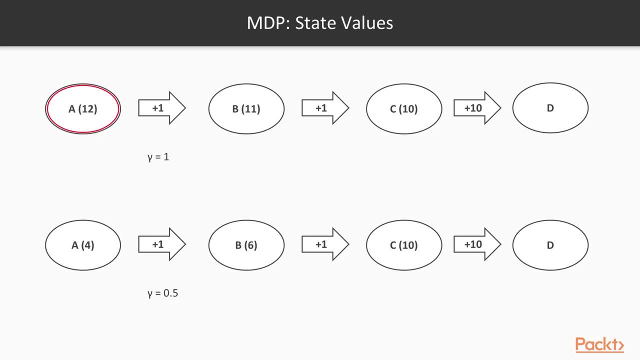 The transition probability at each step is 1, and goes from A to B to C and then stops at. Inside each circle is the name of the state, a letter, and the state value inside parentheses. The top example has gamma equal to 1.. The bottom example has gamma equal to 0.5,.